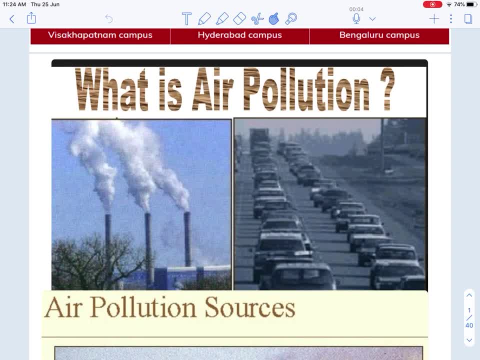 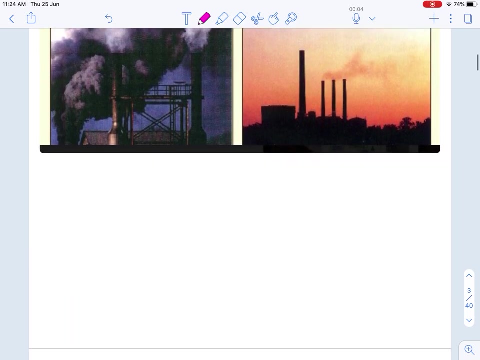 air pollution. If you are living in a city- smoke coming from automobiles, or if you are living in industrial area- thick smoke coming from exhaust- you may think that they are polluting the air. There are different sources. They may be natural or they may be man-made. Once these pollutants 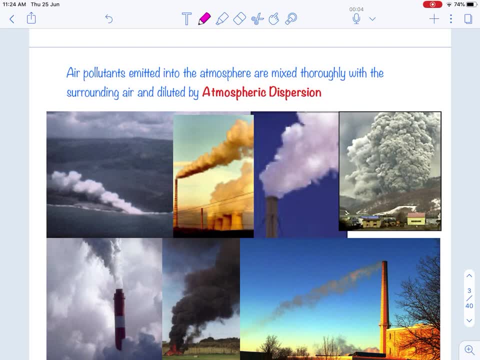 are emitted into the atmosphere, they get diluted, They mix thoroughly with the surrounding air and they are diluted by the term called atmospheric dispersion. So what is dispersion? Dispersion is nothing but spreading of pollutants from a source As they occupy larger and larger volumes of air. they get diluted When a pollutant 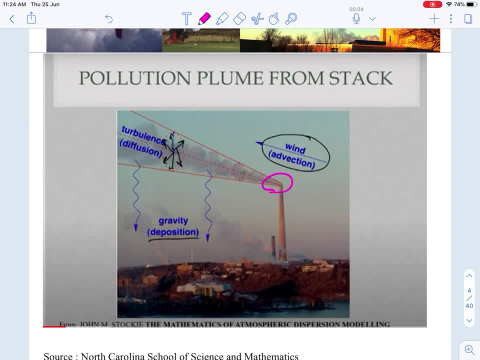 is released from a stack. there are three factors which are responsible for the dispersion. One is the wind. That is nothing, but because of the advection, the pollutant is carried away along the direction of the wind. And secondly, because of the turbulence. because 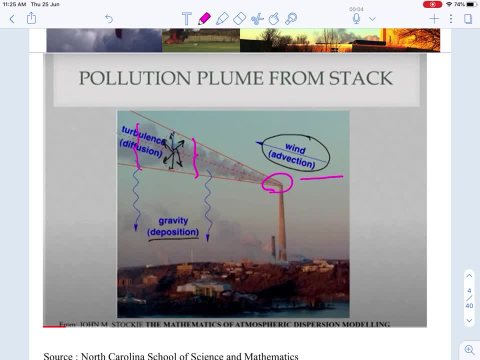 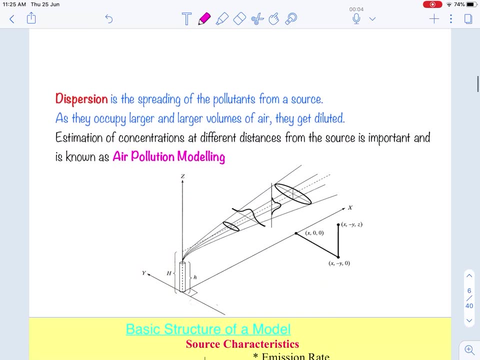 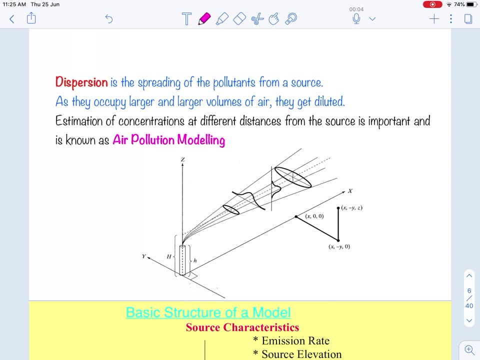 of the diffusion, There is a cross difference in the concentrations. And third, one is gravity deposition, Why we require this air pollution modelling: To find the ground level concentrations for a given source at different points and to compare these with the standards, that is, 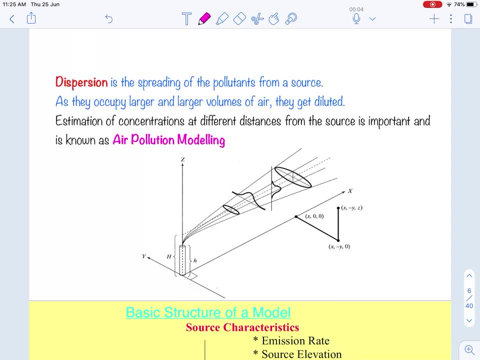 whether they are in the limits or not. And secondly, to estimate the public health of the environment If we calculate the risks associated with the emission of toxic chemicals and hazardous substances, that is, we can calculate the distance up to which the people are at risk. 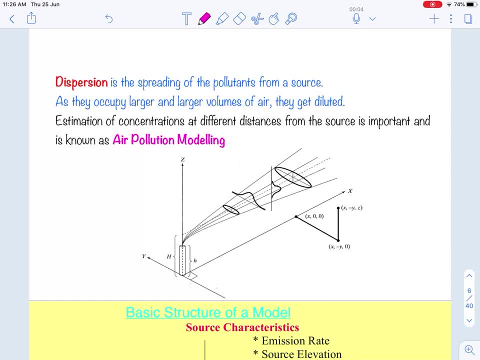 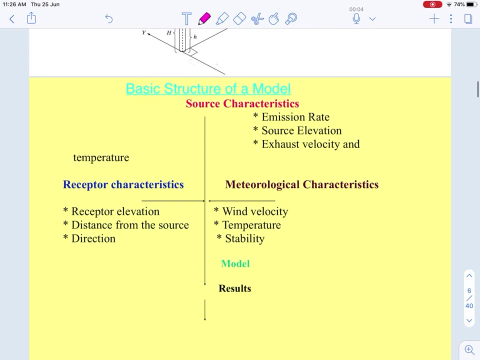 and not only that: to estimate the efficiency of controlling equipment and to plan for reduction measures For any model we require source parameters- metallurgical parameters and receptor parameters, That is, source to experimental and electrical applications. So the risk of pollution is that the people have to go back for the treatment, or at least 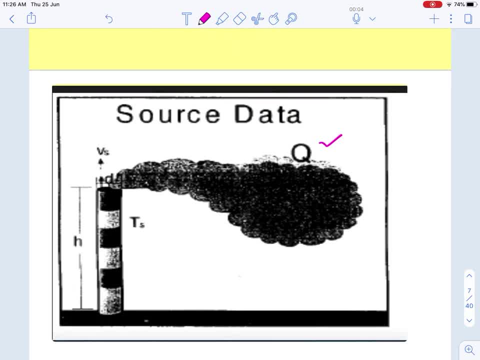 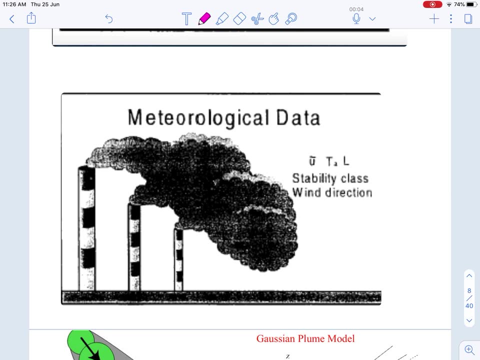 parameters like source emission rate, stack height, temperature, stack exit velocity and the diameter of the stacker. coming to the metallurgical parameters we require the wind velocity, ambient temperature and the stability class. we'll discuss about how the stability class varies with the temperature and with the altitude, and not only that. the third parameter is the. 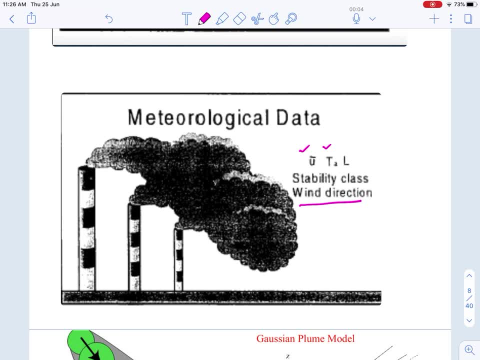 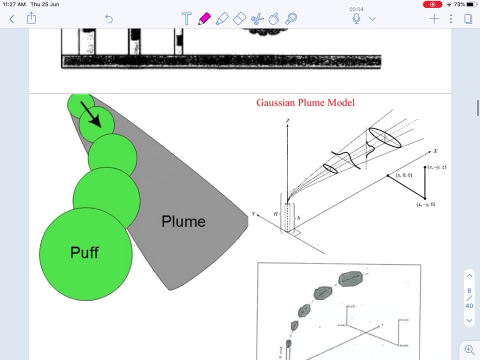 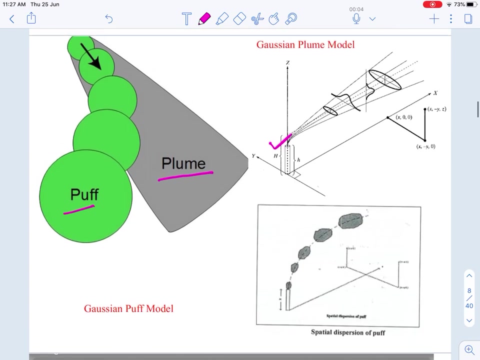 receptor, the receptor elevation, distance from the source and the direction with respect to the source. so here, as far as the air pollution is concerned, there are two sources. one is a continuous source that is coming from a stack, and second is puff, that is nothing but an instantaneous release into the atmosphere, and in this case after time interval. 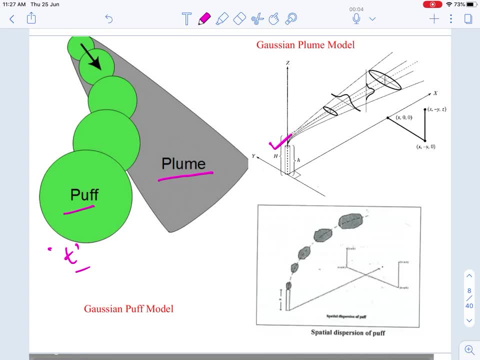 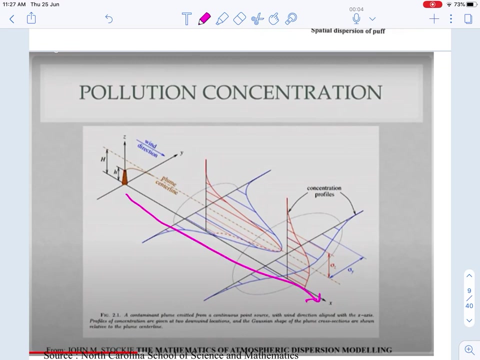 of t, the source becomes zero, but in case of plume it is a continuous source. As far as this, we are following Gaussian distribution and we are following a coordinate system. that means along the direction of the wind, it is x direction, and if you assume that this is the center line of the 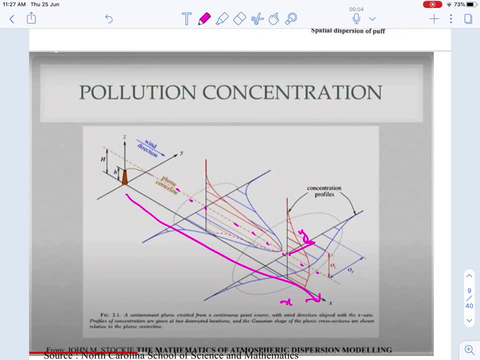 plume away from the center line, that is y, and the vertical direction as z. So in this, if you consider small h as a physical stack height, there is a small plume rise that is designated by delta h. So physical stack height and the plume rise gives rise to the effective. 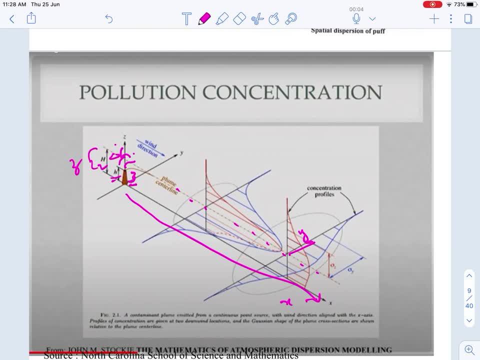 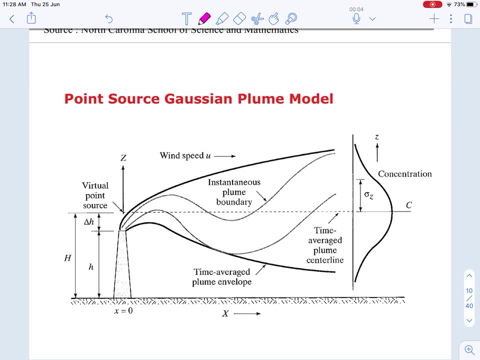 stack height In detail. we will discuss about how to calculate the plume rise And as far as the Gaussian plume model is concerned, that is, firstly, we are concentrating along the direction of the wind as x, and if you assume that this is the center line away from the 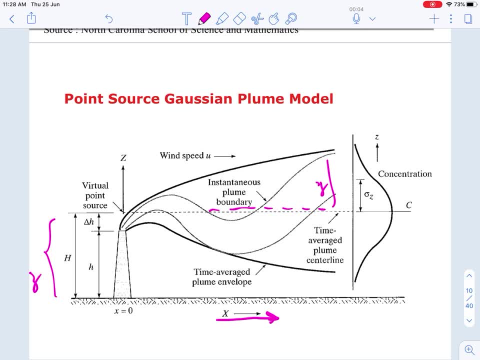 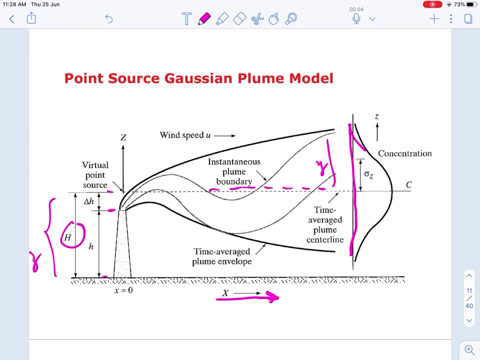 center line, this is y and the vertical distance as z. So this is nothing but the physical stack height, and this is the plume rise. So gives rise to the effective stack height. If you consider the concentrations, it follows a Gaussian distribution that is at the peak at the center and gradually it tapers off. So how to? 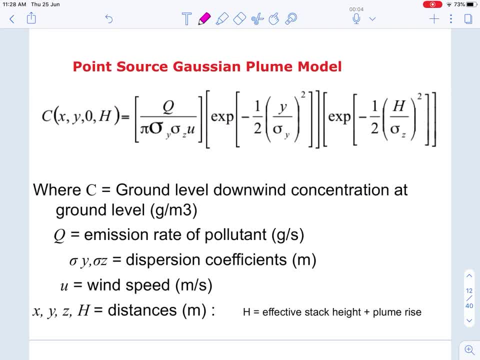 calculate the concentrations. So Gaussian plume model that is, concentration it is. it can be calculated by using this formula. In this q is nothing but the source emission rate. that is the pollutant. how the pollutant is discharged, how many grams per second it is discharged into the 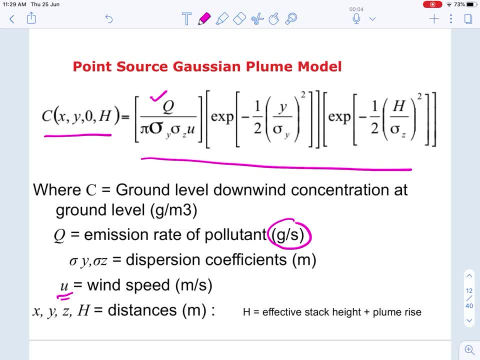 atmosphere. U is nothing but the source emission rate. So this is the source emission rate. So this is the wind speed at the source. x, y, z and h are nothing but the coordinates, and sigma y and sigma z are nothing but the dispersion coefficient in y and z direction. We'll discuss about how to. 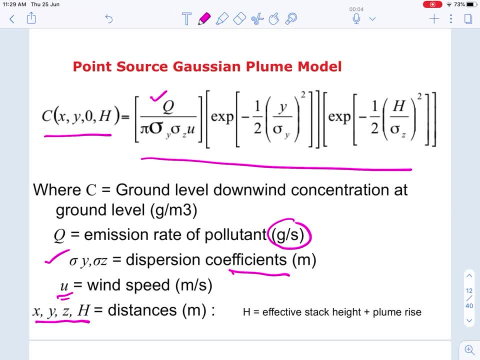 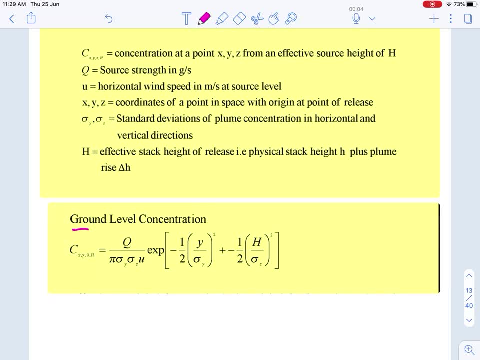 calculate this sigma y and sigma z. See, our interest is how the concentration, ground level concentration- is varying. So if you, if you're talking about the ground level concentration, that means z is equal to zero. So if you substitute the ground level concentration, z is equal to zero. This is the equation for calculating ground level concentration. Now 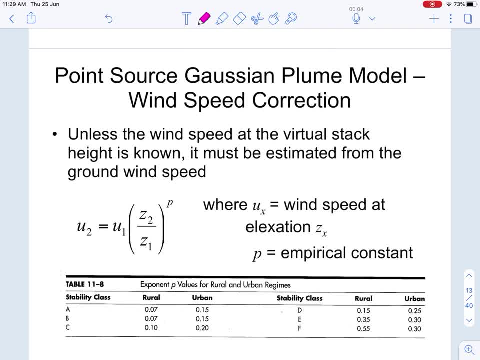 there is a small correction factor, even for the wind. Wind velocity also changes with altitude. Usually the wind velocity is measured at 10 meters height. That is all. the meteorological parameters will measure at 10 meters height. So if you know the wind velocity at a particular 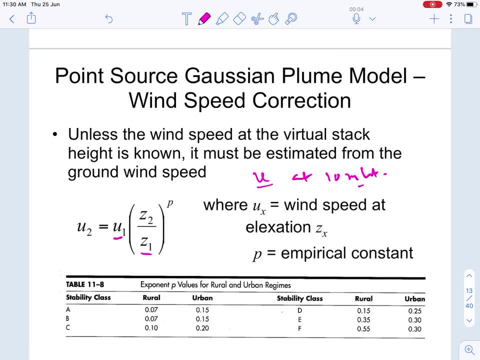 distance, then you can calculate the wind velocity. So if you know the wind velocity at a particular distance, z 1, you can calculate. for example, u 2 is nothing but your stack height You can calculate. z 2 is nothing but your stack height. You can calculate the velocity at the stack height by: 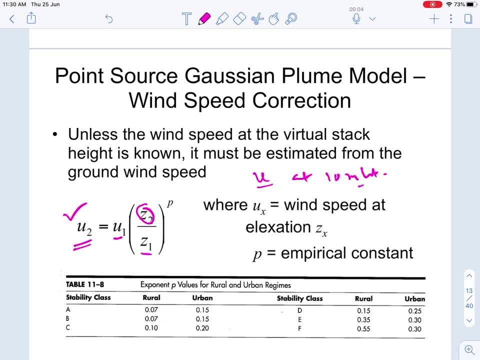 using the formula, u 2 by u 1 is equal to z 2 by z 2, z 1 whole to the power of p. P is nothing but the empirical constant depends on whether it is rural or urban, etc. So this correction factor, we 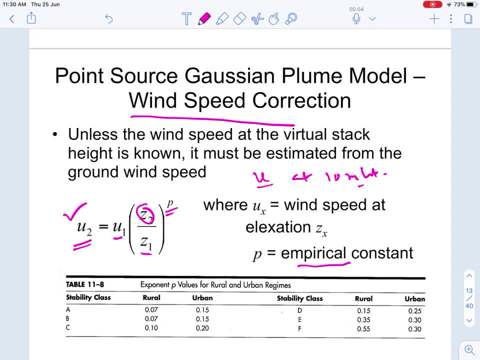 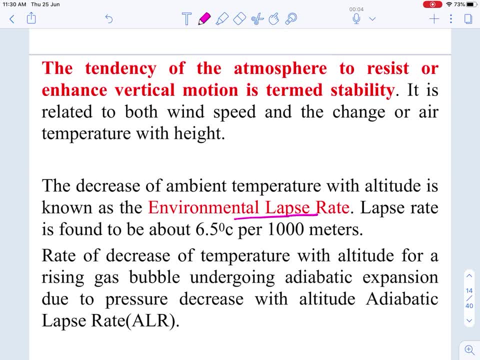 can use it to find out the exact wind speed. At the stack exit there is a term called environmental lapse rate, That is, the temperature is decreasing with the altitude. So that is nothing but the environmental lapse rate. Usually it is found that 6.5 degrees centigrade decrease of temperature for every thousand meters. 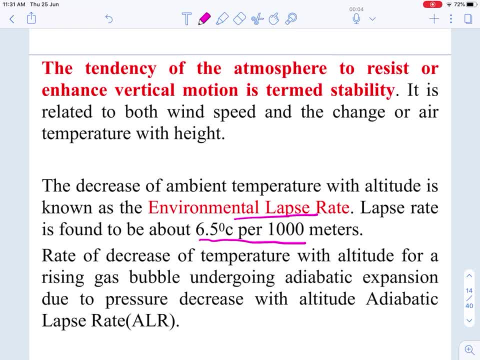 So when a parcel of air is released into the atmosphere because of the decrease in the pressure, because of the temperature, because of the expansion, It goes adiabatic expansion and it also reduces the temperature. That is called adiabatic lapse rate. 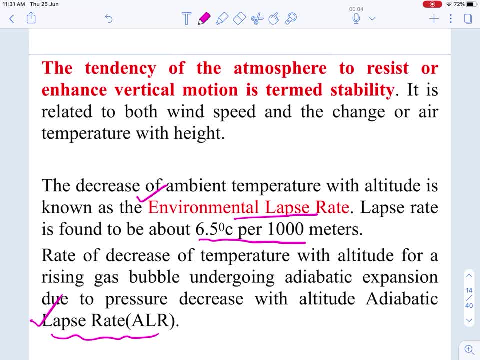 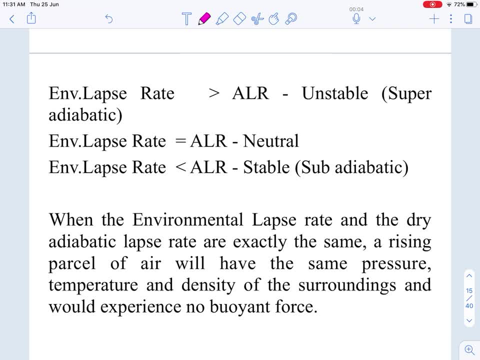 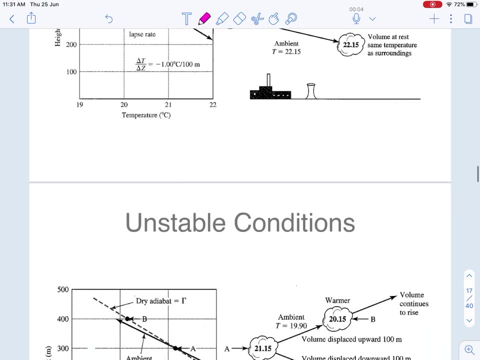 So when you compare this environmental lapse rate and adiabatic lapse rate, we can classify the atmosphere into different stability conditions, For example, when environmental lapse rate is greater than adiabatic lapse rate. What do you mean by that? When it is environmental lapse rate, 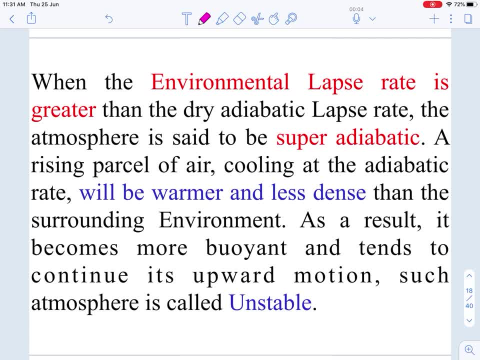 is greater than the dry adiabatic lapse rate, That is, the atmosphere is cooling faster than a parcel of air. So a parcel of air is cooling. it is more warmer than the surrounding and less dense. As a result, it becomes more buoyant and it tends to continue in the upward direction, So that stability. 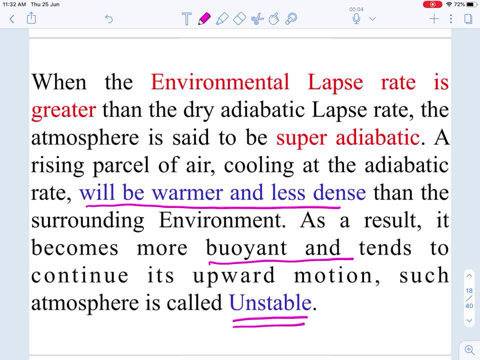 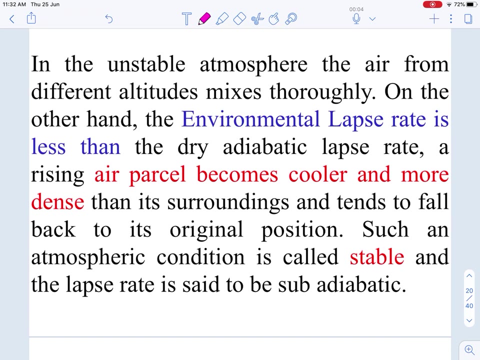 condition is called unstable condition. This is when the environmental lapse rate is greater than the adiabatic lapse rate, The condition it is called super adiabatic and the climatic condition: it is designated as unstable. And there is another term when it is on the negative side, That is, when the 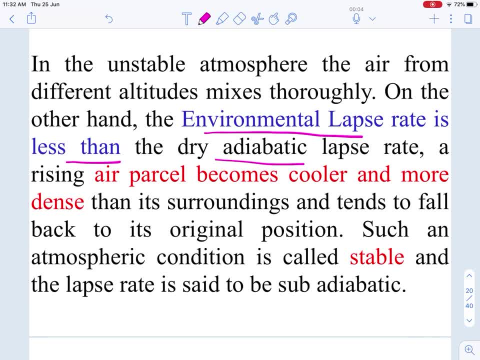 environmental lapse rate is less than the dry adiabatic lapse rate. That is a parcel of air coming from a stack. It becomes cooler and more dense than the surrounding. As a result, what will happen is that it falls down to the ground. it falls down to the original. 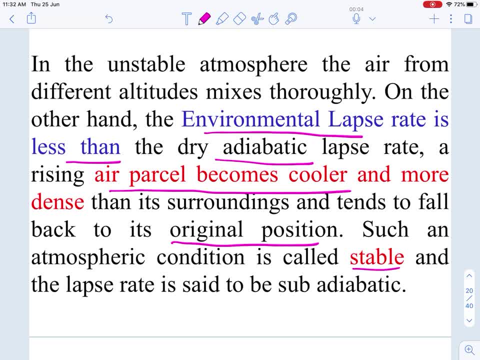 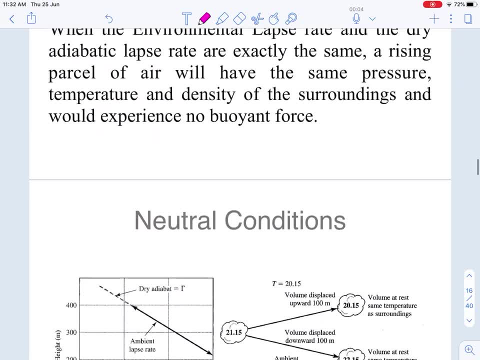 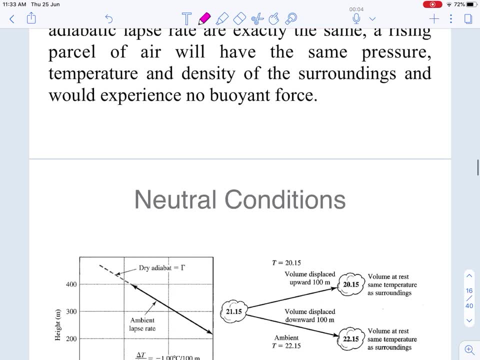 position. As a result that atmospheric condition it is said to be stable when environmental lapse rate and the adiabatic lapse rate are both the same, then we will call the neutral condition. But that means there is no much influence on the temperature, on the climatic condition. 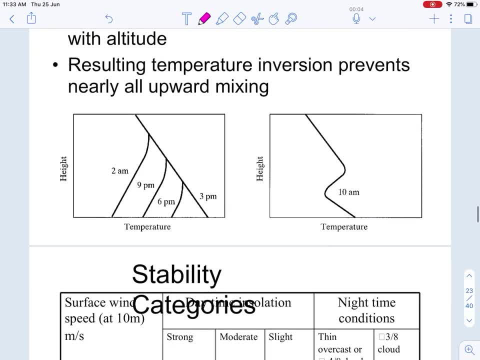 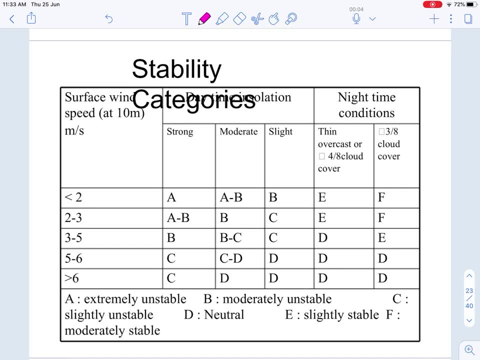 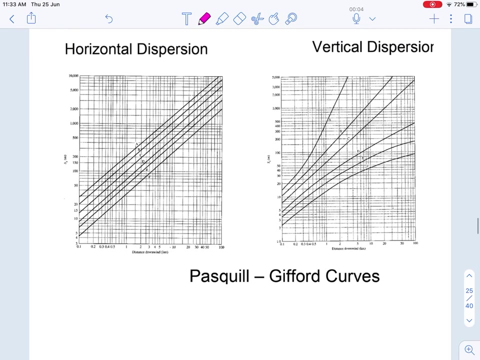 So Pascal and Gifford. they have classified based on the temperature, based on the solar in radiation, they have classified the climate conditions into extremely unstable, moderately unstable, slightly unstable, neutral, slightly stable and moderately stable condition. so these readymade pascal and gifford curves are available. 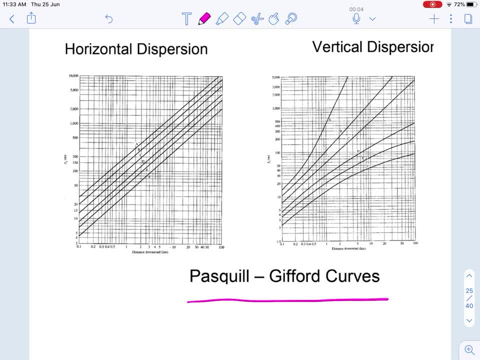 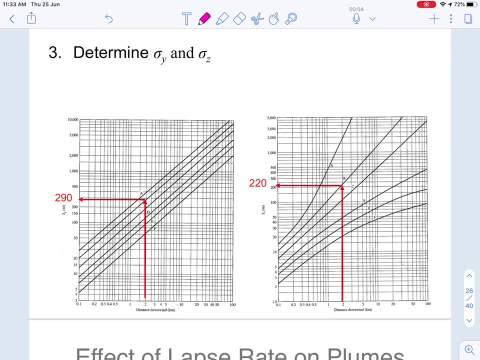 so we'll, i did. we'll- find out how to calculate the dispersion coefficients, sigma y and sigma z. see, for example, if my distance is, let us say, two kilometers. so, correspondingly, if i am choosing any climatic condition, so i can calculate, i can read the sigma y value. similarly, i can calculate, i can. 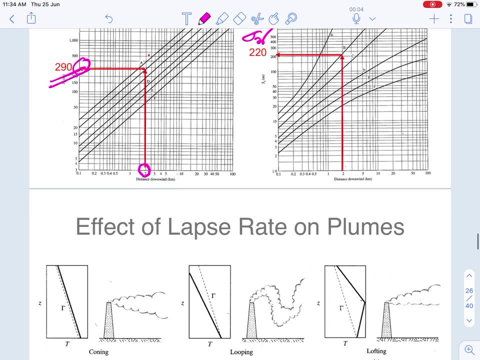 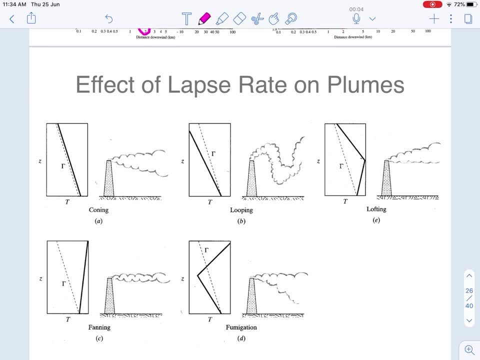 read the sigma z value from this readymade curves. so, based on the climatic conditions, the plumes, they behave in different ways, that is, coning, looping, fanning, fumigation, etc. in another video we'll discuss about how this plume behaves with respect to the 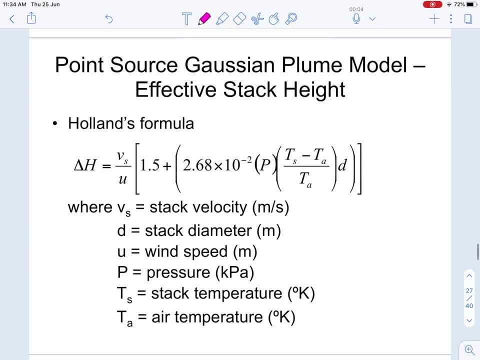 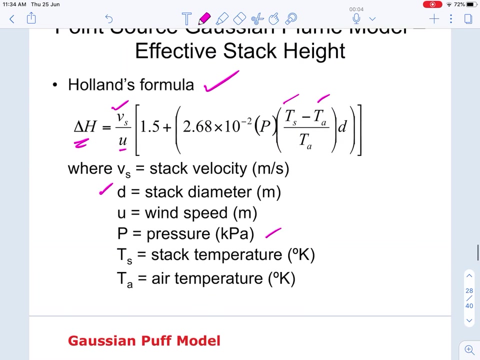 lapse rate. so this is a formula for calculating the stack height. it depends on the stack exit velocity, diameter of the stack, wind velocity, atmospheric pressure, stack exit temperature and the ambient temperature. this is called whole and formula. so we'll calculate the delta h and we know the physical stack height. then we'll calculate the effective stack height. 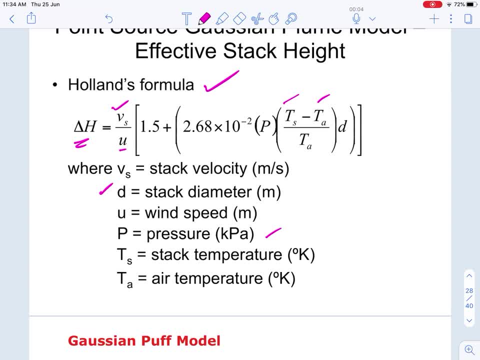 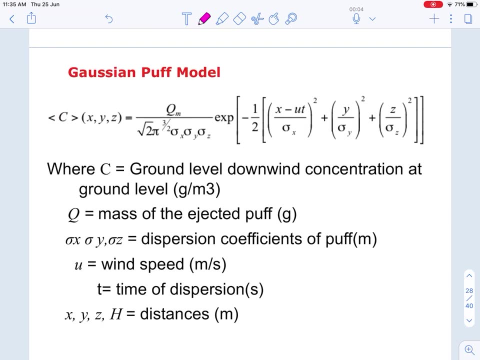 then we'll correct the velocity at the source, then suitable climatic condition we'll choose. depending on that we will calculate sigma y and sigma z. then all these are the input parameters to the ground oil concentration. Coming to the second part of the model, that is, Gaussian puff model, as 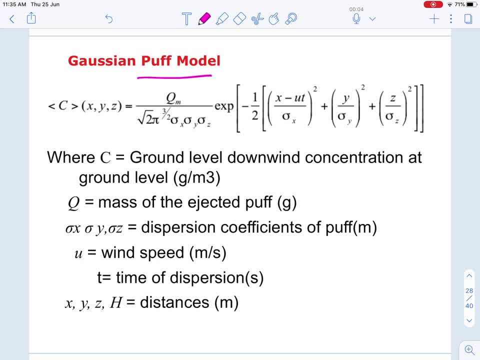 we have already mentioned that puff pins, it is nothing but an instantaneous release into the atmosphere. that is, after a particular interval of time, t, the source becomes zero. So in this, how much mass of pollutant is injected into the atmosphere? so many grams? and sigma x, sigma y and